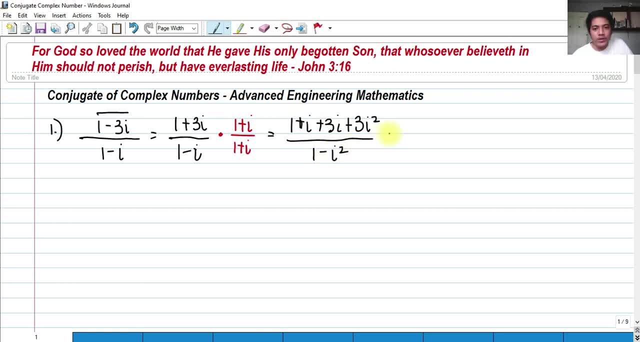 term And that is all over 1 minus 3i. And then evaluate, So we have 1 plus 4i. 3i plus i is 4i. We know that i squared is equal only to negative 1.. So might as well we have the substitute negative 1.. So we have negative 3 plus 1 is. 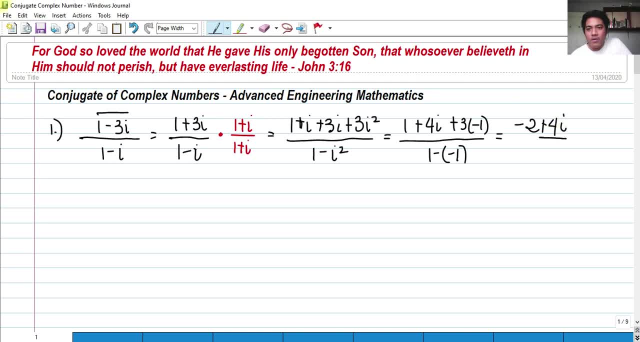 negative 2. That is plus 4i. all over 1, minus negative 1 is 2.. So we can further simplify this. We can factor out 2.. We have negative 1 plus 2i. okay, all over 2 times 1.. Okay, so we cancel 2.. Then we have an. 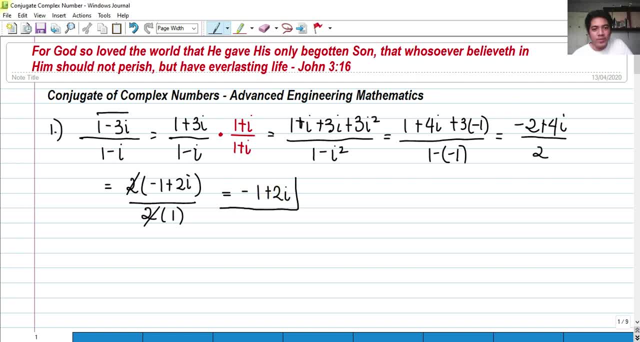 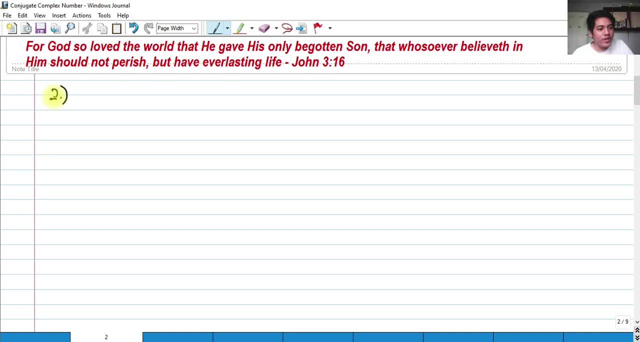 answer finally: negative: 1 plus 2i. So this would be our answer for our problem, number 1.. So for number 2, let's try again to solve. Our given is the conjugate of 1 minus i, all over i plus. 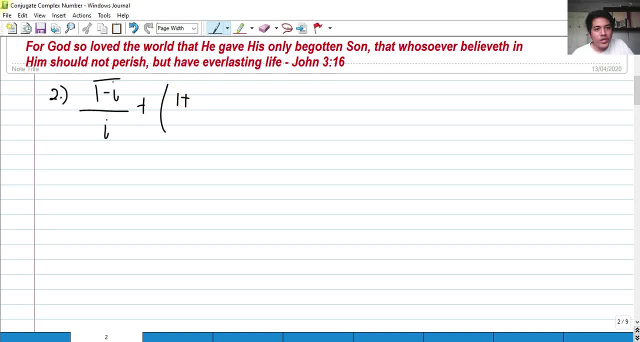 quantity: okay. conjugate of the whole term: 1 plus i. all over i. Okay. so how are we going to evaluate? So this is the conjugate of the whole, including the numerator and the denominator. So first we need to evaluate the conjugate of the numerator. for the first term, We have 1 plus i. 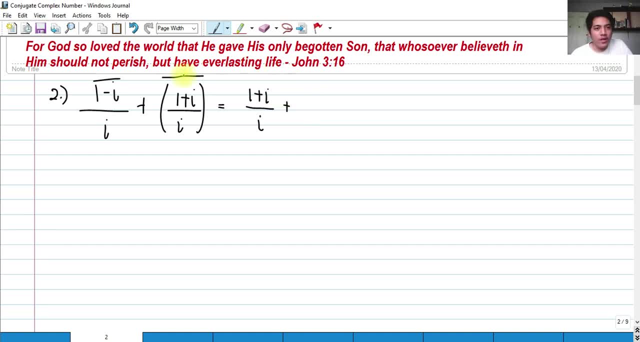 all over i- okay, and then plus properties of conjugate. we can distribute this on the numerator and the denominator. So what we're going to do is simply we have 1 plus i- conjugate- okay, and the conjugate of i on the. 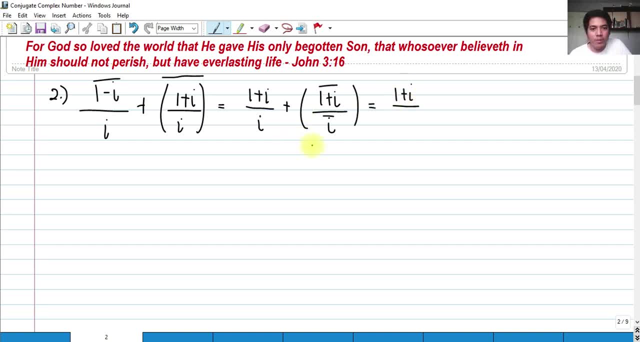 denominator and evaluate its conjugate. That's one property of conjugates. So we have 1 minus i- okay, all over. we have negative i Okay. so again, in order for us to solve this, we need first to eliminate the i on each of the denominators. So we'll be having 1 plus i- all over i plus i, all over i. 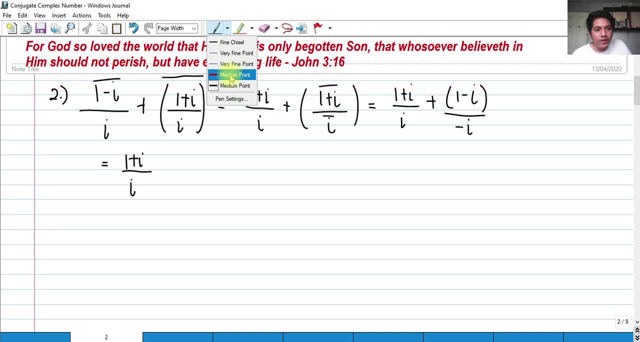 And this would be multiplied. This would be multiplied To the conjugate of its denominator, negative i, for the first term, And then we have 1 plus i, all over negative i and the conjugate of negative i should be negative i or positive i. I mean, So positive i over. 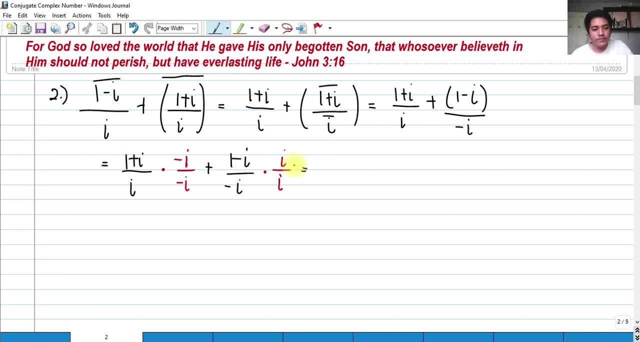 positive i, And then it okay. so what are we going to do here? simple numerator, times numerator, denominator, times denominator. so we have negative I minus, I squared all over. negative I squared. that is plus here. we have I minus, I squared all over. we have negative I squared, but I squared, as we all know, that's equal to negative one. 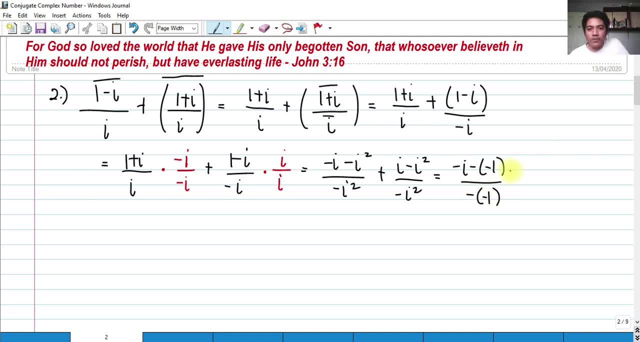 all over negative, negative, one plus. we have I minus negative one. then we have negative of negative one. so, as you can see, the denominator is only equal to one, so we can rewrite this as I plus one or one minus I, this one plus, then we have one plus I, one plus I. so if you're going to evaluate this, one plus one. 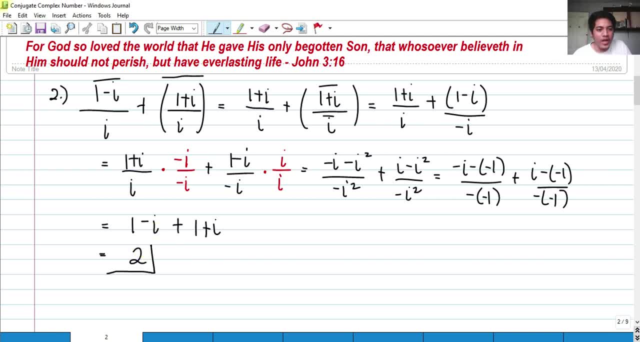 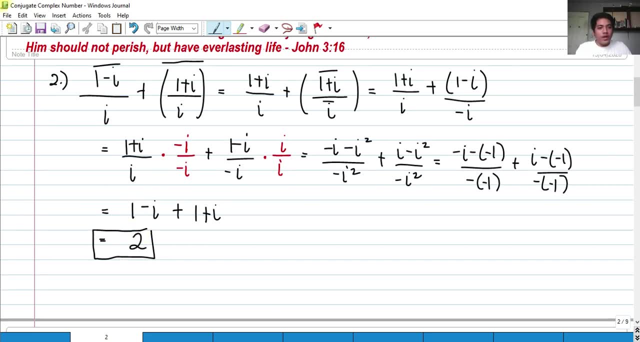 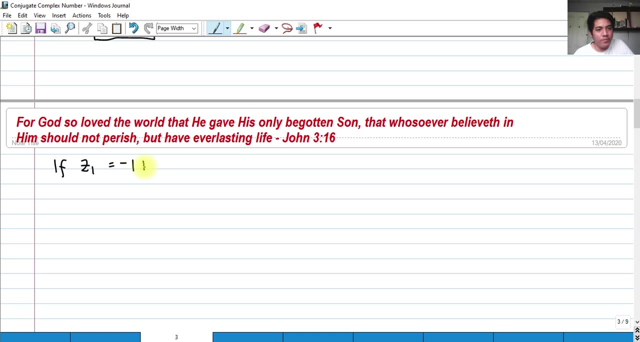 that's two negative I plus I, would be cancelled. so we hence we have an answer that is equal only to two. okay, let's proceed with number three. so proceed first with the given. if Z of one is equals to negative, one plus I, and Z of two is equal to two minus three I we're going to evaluate number three, quantity. 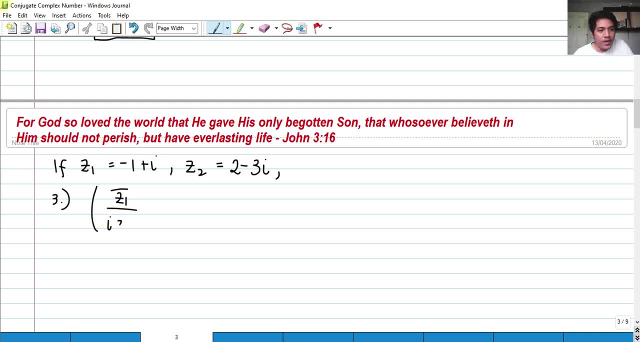 conjugate of Z sub one over I times Z sub two. okay, so first we're going to get the conjugate of Z sub one. so Z sub one conjugate would be negative one minus I, all over. I multiplied by Z sub two, two minus three, I, so I evaluate negative one. 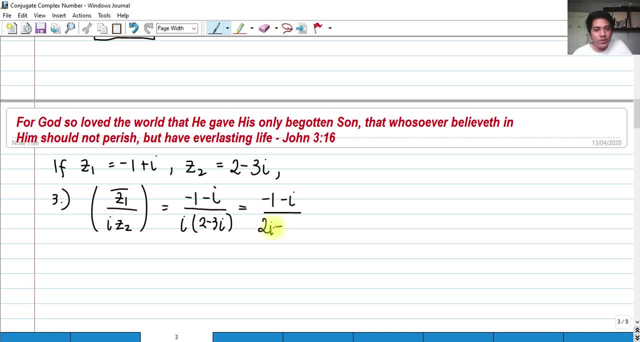 minus I. so we have two I minus three I squared and evaluate the I squared. two I minus three. two I minus three times negative one. okay, so we have now negative one minus I. this would be positive three plus two I. okay, then we're going to evaluate this by multiplying it by the conjugate of the. 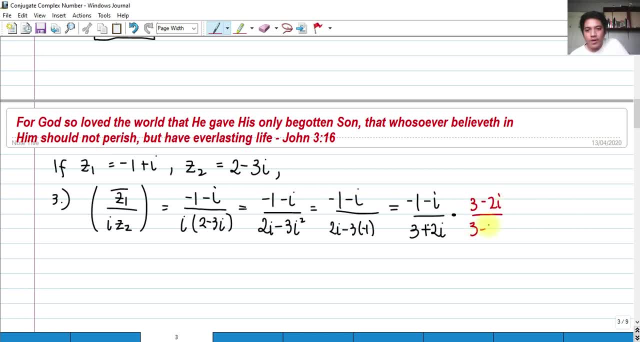 denominator: T minus two I over T minus two I. so simple again, simple multiplication of fractions. so we have negative three, that's the first. the outer is plus two I. the inner is negative three, I. and the last one is positive two I squared. okay, let me just 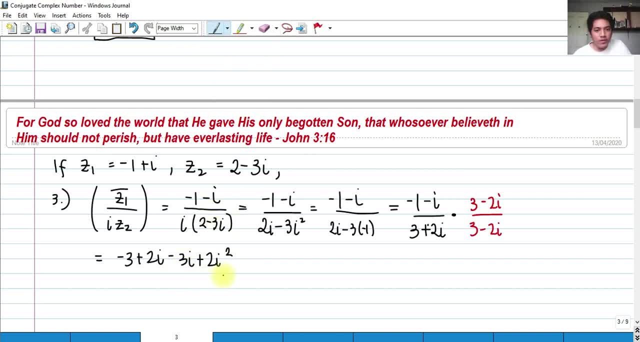 rewrite this: two- I squared. all over. we have nine I minus four I squared. evaluate this: I squared. so first simplify this. we have negative three, two I minus three I, that's minus I, we know that- plus two times negative one. and then we have nine minus four times negative one. okay, so we. 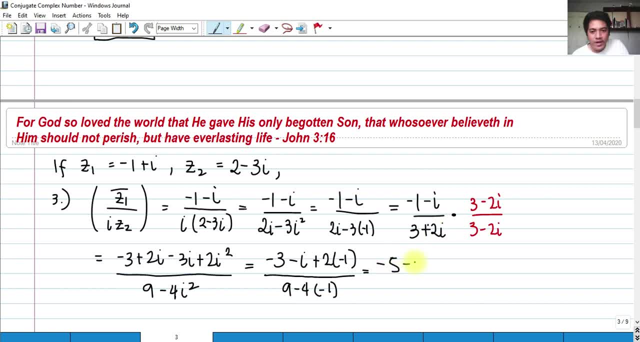 have now negative two minus three, that's negative five minus I, okay. and then we have nine plus four, because this becomes plus because of the negative one, that's 13. so our answer would be negative: five over 13 minus one over 13 I. so this: 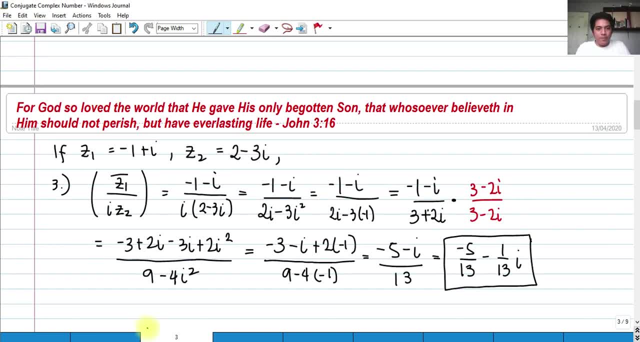 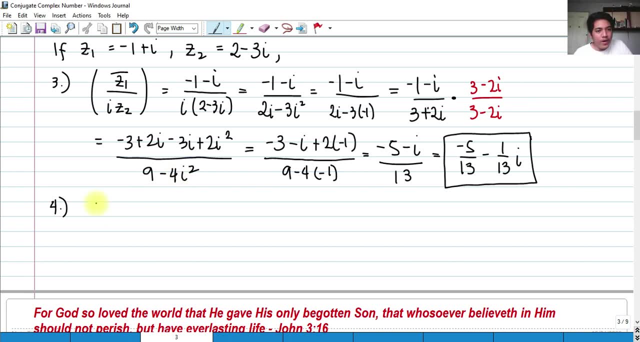 should be our answer for this problem. number three. for number four, okay, let's try to have another problem we have. I, multiplied by the conjugate of Z is of 1 all over Z sub 2 minus I. okay, going back to our given, these are our given I. 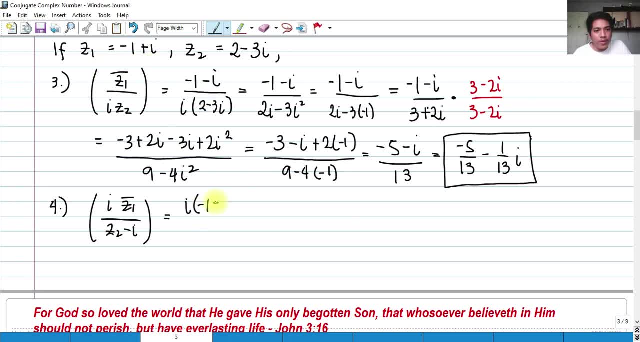 multiplied by the conjugate of Z sub 1 as negative: 1 minus 1, all over the Z sub 2, 2 minus 3. I multiplied by or minus I minus I. so we have negative I minus I, squared all over, we have 2 minus 4 I, but we know that I squared okay is equal. 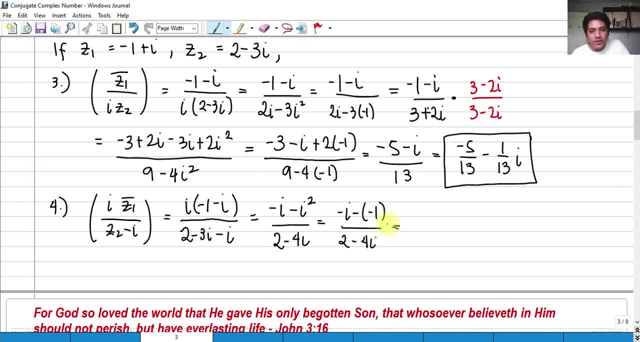 to negative 1. okay, in that's this would become 1 minus I, all over, 2 minus 4i. all right. and then, finally, we saw this: by multiplying in Y- it's conjugate, the denominators conjugate- we are 2 plus 4i. 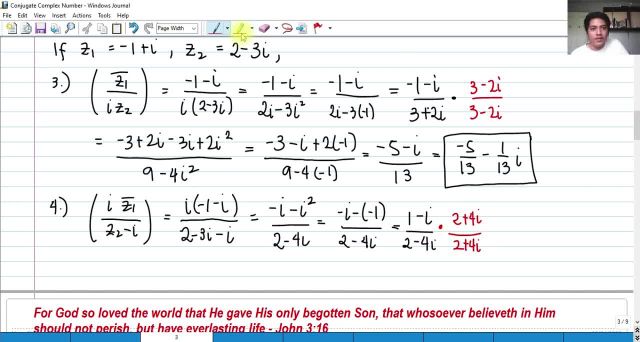 all over 2 plus 4i. i then evaluate. so you need to evaluate that. so first we have two outer, we have plus 4i, inner we have minus 2i and last term we have negative 4i squared and that is all over 4 minus 16. okay, i squared, okay, and evaluate this simplify. 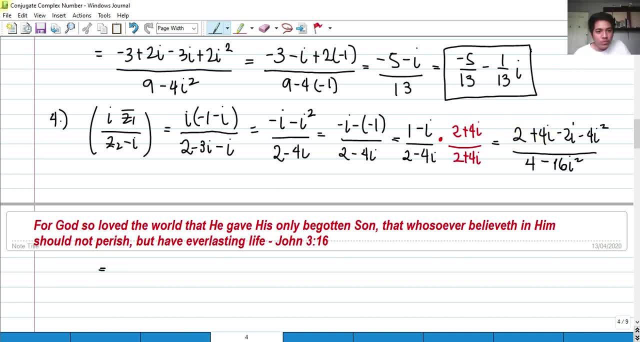 this. so we have uh 2, then we have 4i minus 2i, that's plus 2i. then we have negative 4 times negative 1, all over 4 minus 16 times negative 1. so this would become plus 4 plus 2, that's 6 plus 2i. 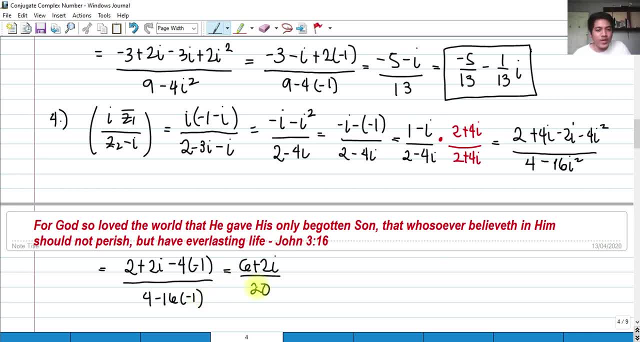 all over 20.. okay, 20.. okay. so we can further simplify this by factoring 2. we have 3 plus i. all over, we have 2 times 10, so the 2s will cancel. so we have a result as 3 plus i over 10, or 3 over 10 plus 1 over 10 i. this should be the result of our problem number 4.. 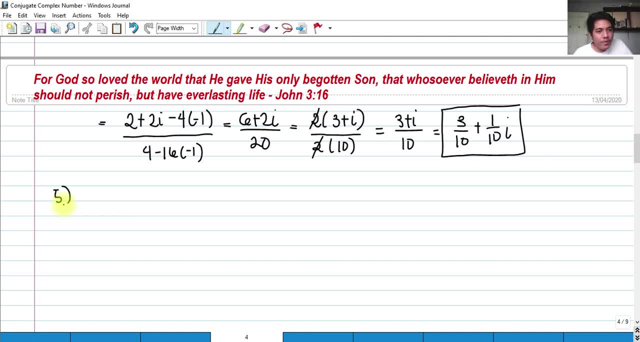 so let's go now to problem 3, problem number 5. for problem number 5 we have conjugate of z sub 1 all over z sub 1 plus z sub 2, plus quantity conjugate of z sub 2 all over z sub 1 plus z sub 2. 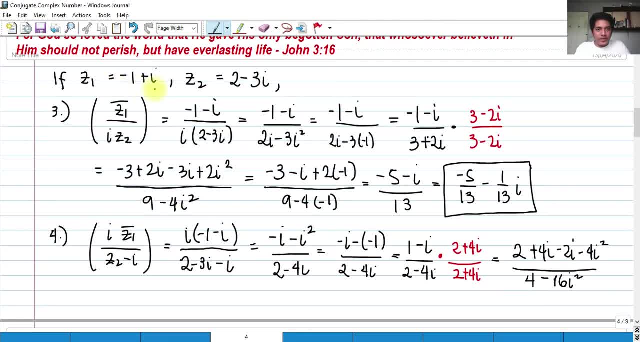 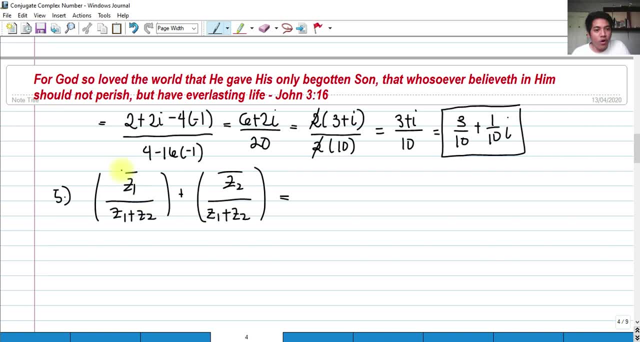 so, going back to our given, okay, we have this given: negative 1 plus i, then z sub 2, 2 minus 3 i, so we're going to substitute it. the conjugate of z sub 1 is actually negative 1 minus i. that is all over. j sub 1 plus j sub 2. we have negative 1 plus i, negative 1 plus i, and that is. 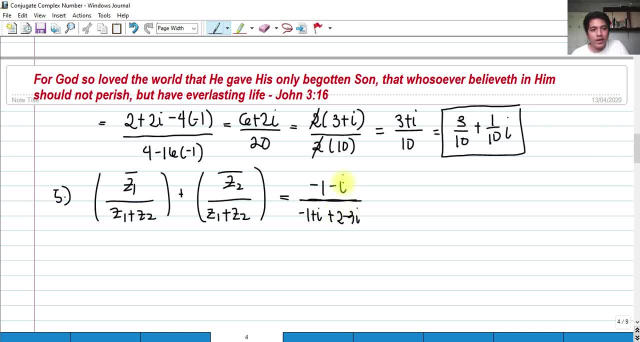 plus 2 minus 3 i- okay for this term- and then plus the conjugate of j sub 2, that's 2 plus 3 i, and then we have the same for the denominator, and then we have the same for the denominator, and then we have. 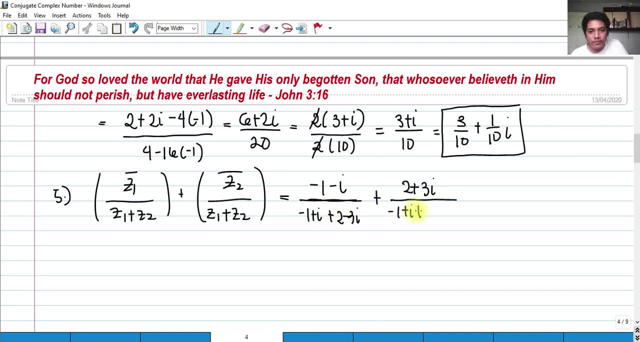 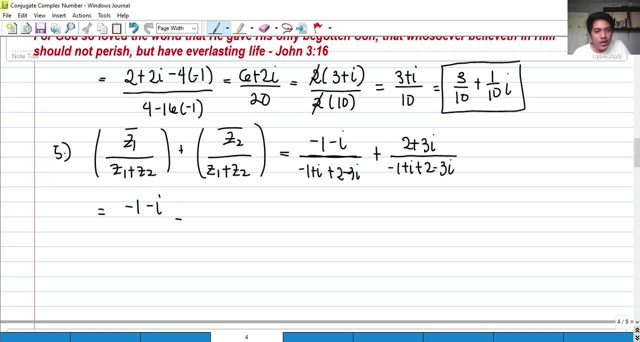 the same for the denominator as the first term, okay. so what are we going to do here? simplify: negative 1 minus i. so we have negative 1 plus 2, that is 1- okay. then we have i minus 3, that's 1 minus 2, i okay. and the same for this: 2 plus. 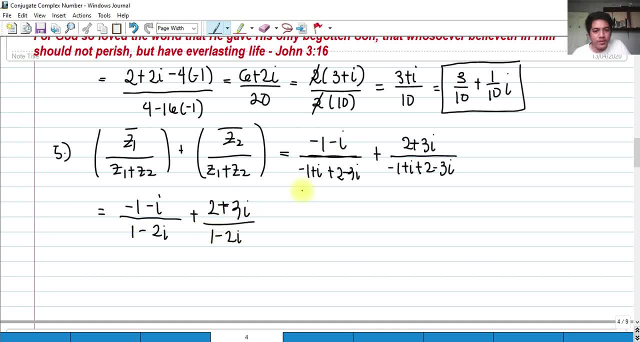 3: i the same for the denominator, so we can combine this because they have the same denominator in both. so plus 3i. so we have this because they have the same denominator. so we can combine this because they have the same denominator as be Maick'if. 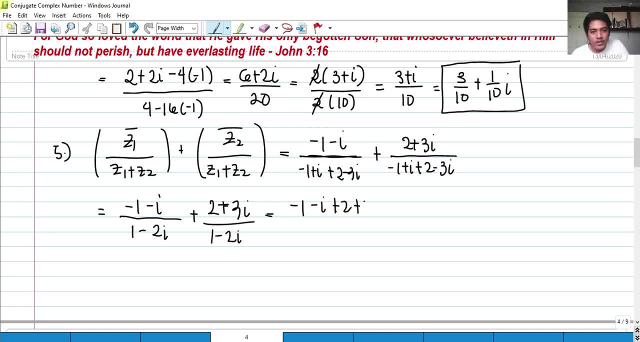 negative 1 minus i plus 2 plus 3i, all over 1 minus 2i. simplify: and then we have negative 1 plus 2, that is 1 negative i plus 3i, that is plus 2i all over 1 minus 2i. and of course we're not yet done. 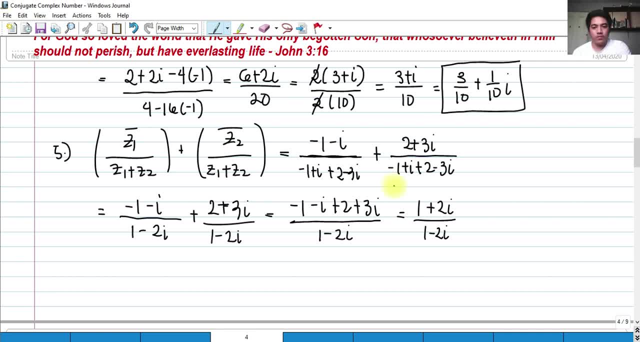 we're going to multiply this, as we know, by the conjugate of the denominator. so we have multiplied by 1 plus 2i over 1 plus 2i, so we have an answer of 1 plus. we perform the foil of this. our answer should be 1 plus. 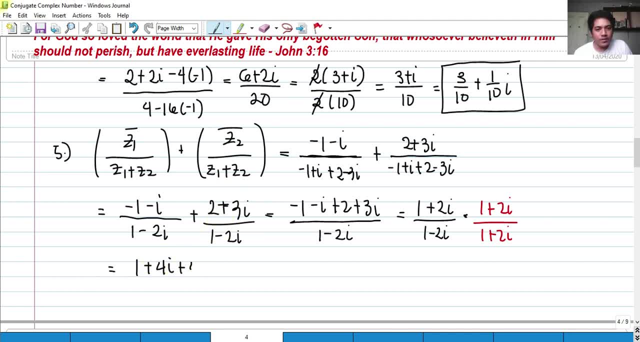 1, four. i plus four: i squared all over. one minus four: i squared okay. then we have to evaluate the i squared as negative one. then we have this answer. so we have one minus four. that's negative. three plus four: i all over, we have five okay. 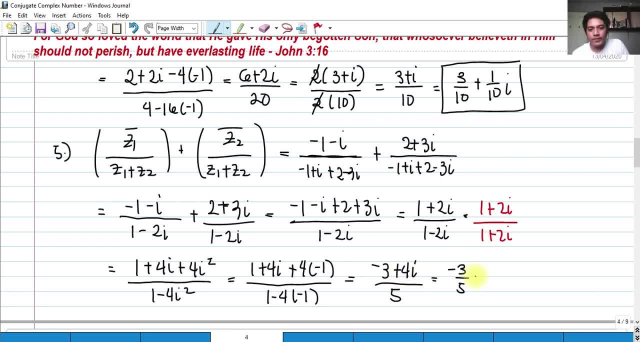 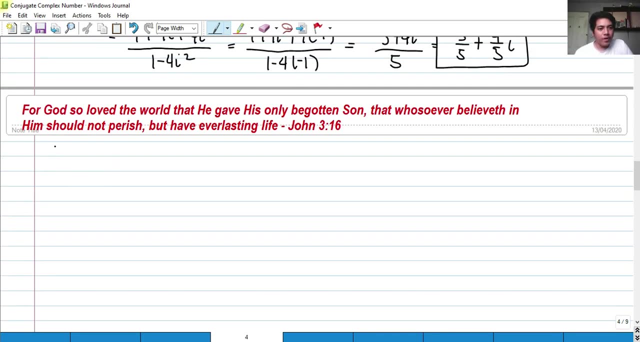 so. So our answer should be negative: 3 fifths plus 4 fifths of i, and that is our answer for this problem. So let's try another problem. okay, For number 6, if z sub 1 is equal to 1 plus i and z sub 2 is equal to 2 minus 2i, 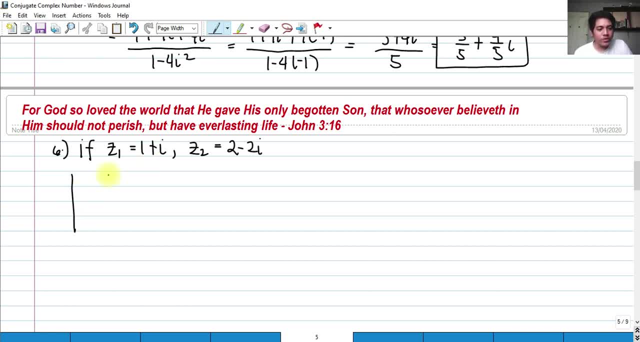 then we're going to evaluate the modulus of 1 minus z sub 2 over the conjugate of z sub 2 minus 1.. Notice that we have now a modulus, So our answer should be a real number, positive real number. okay. 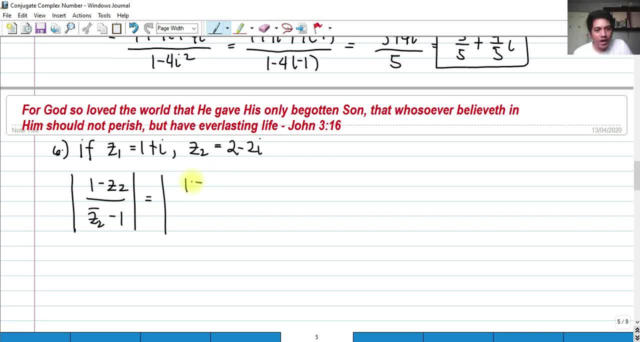 So we have first we have 1 minus z sub 2, that's 2 minus 2i. Be careful with the minus sign. You have to Distribute that. The conjugate of z sub 2, that's 2 plus 2i minus 1, okay. 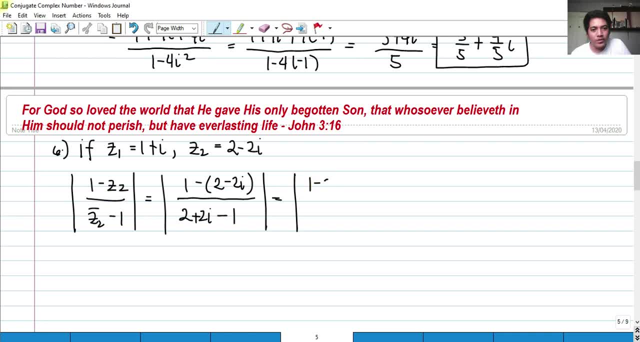 So what will happen here is we have 1 minus 2, okay, Plus 2i, all over 2 minus 1, that's 1 plus 2i, the modulus of that, And of course, if we simplify this, that is negative: 1 plus 2i, all over 1 plus 2i. 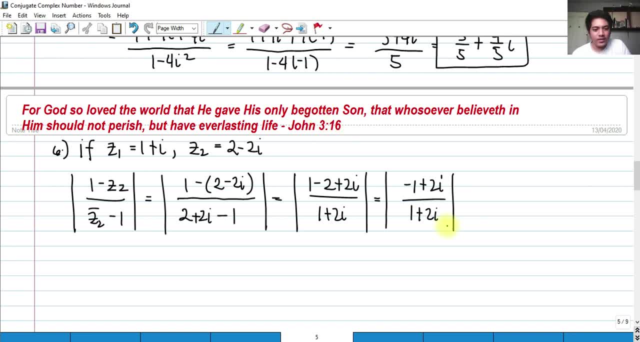 And we know what to do with this. in order for us to evaluate this, We need to multiply this by the conjugate again of the denominators. So what will happen here is we have 1 or negative, 1 plus 2i, all over 1 plus 2i. okay, 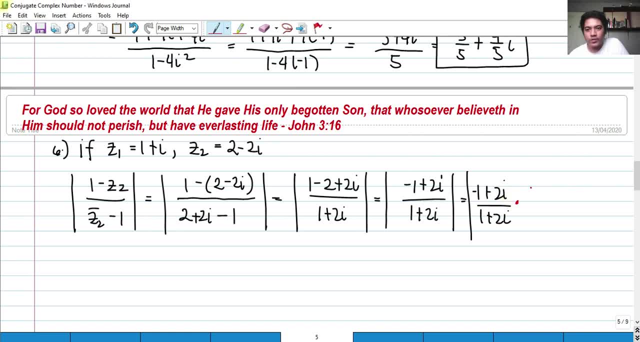 And then we have to multiply it by the conjugate, So we have 1 minus 2i. all over 1 minus 2i. Don't forget the modulus. Okay, Evaluating that. so we have negative 1, okay. 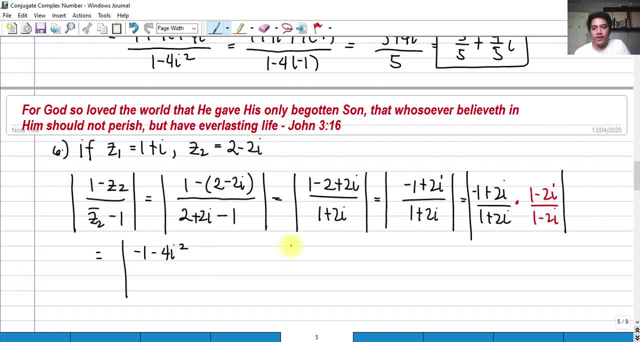 And then minus 4i squared, because this is a difference. okay, I know, We have to evaluate it, because this is negative 1 and this is 1.. They are not entirely the same, So we have to perform still the Paul method. 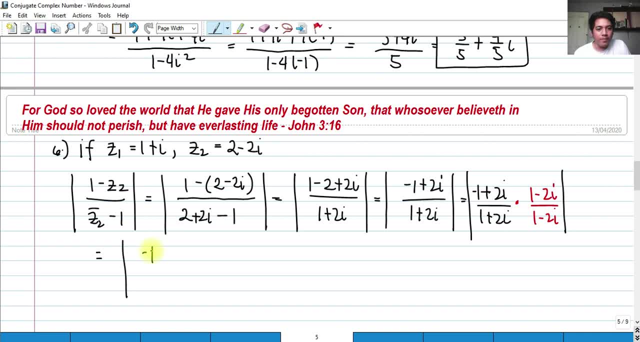 So we have negative 1, first, Outer. we have plus 2i. We have inner, okay, That's plus 2i. Then we have the last, That's negative 4i. squared All over, okay, This is only difference. 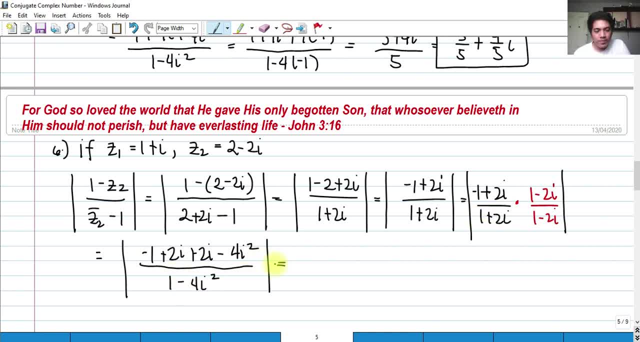 So we have 1 minus 4i. squared Simplify. So we have negative 1.. We have 2i plus 2i, That's 4i. Then we have minus 4 times negative 1.. On the denominator, we have 1 minus 4 times negative 1.. 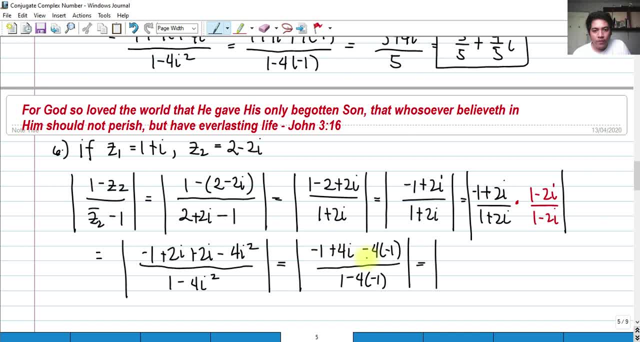 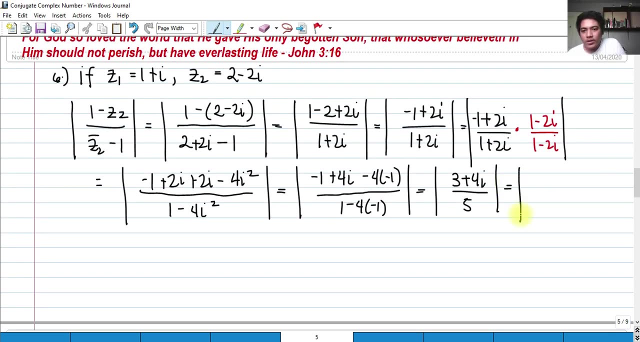 So we have 4 minus 1.. That's 3 plus 4i All over. this should be 5, okay, The modulus of 5.. So, in order for us to get the modulus of that, so we can rewrite this as 3 fifths plus 4 fifths i. 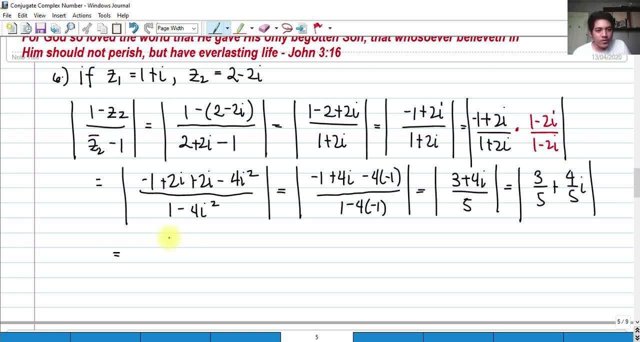 So we know that this is our x, This is our y In order for us to get that. so we have to square x, Okay, plus the square of y. Then we square it out, okay. So what will happen here is that we have 9 over 25 plus 16 over 25.. 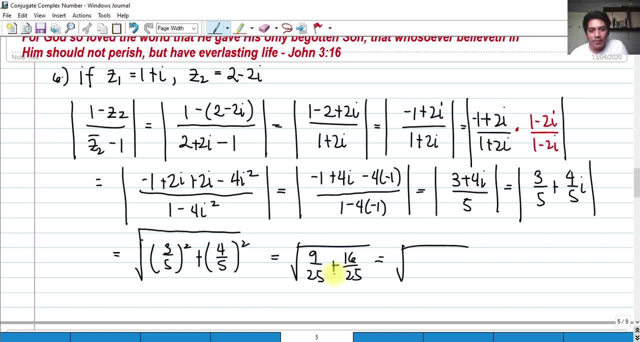 So 9 plus 16.. So we can add this, because they have the same denominator 25.. 9 plus 16 is 25 over 25, of which we know that that should be the square root of 1.. And the square root of 1 is only equal to. 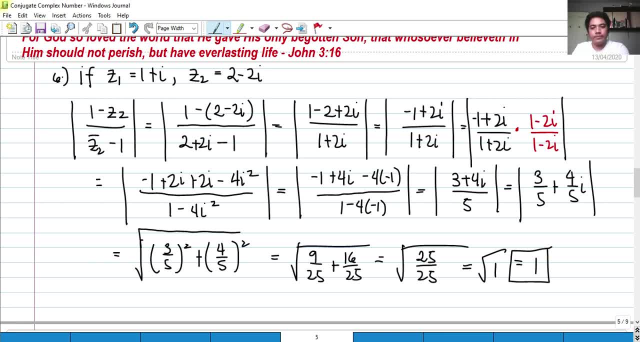 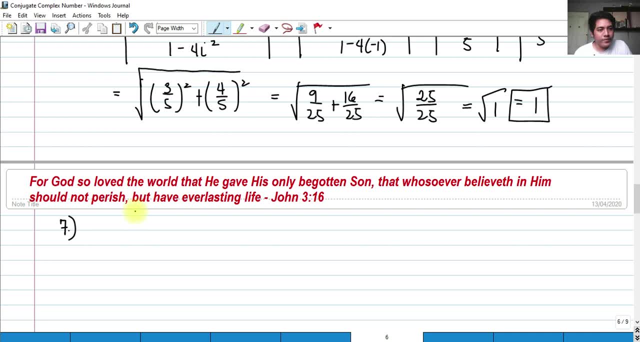 1.. And that's our answer for this problem. Okay, let's get another problem, number 7.. So we have 1, half multiplied by the modulus of z sub 1, all over the conjugate of z sub 1.. Okay, let me just rewrite this. 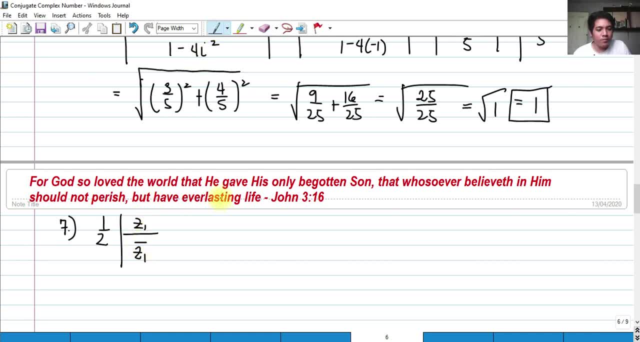 So we have z sub 1 all over the conjugate of z sub 1, plus conjugate of z sub 1 all over z sub 2.. Take the modulus of that, multiply it by 1 half. So first, before we multiply 1 half, 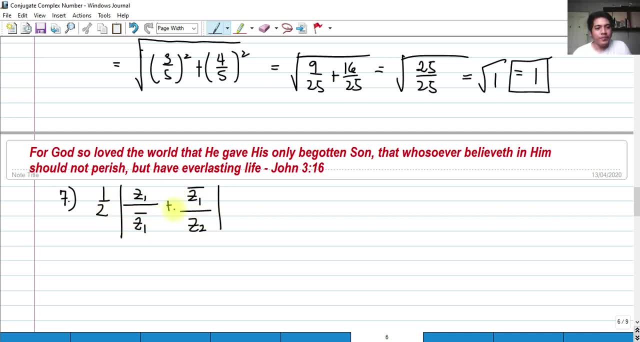 we need to evaluate this inside of the modulus. Okay, so we have 1 half multiplied by z sub 1, our z sub 1,, 1 plus i, all over the conjugate of z sub 1, that is 1 minus i. 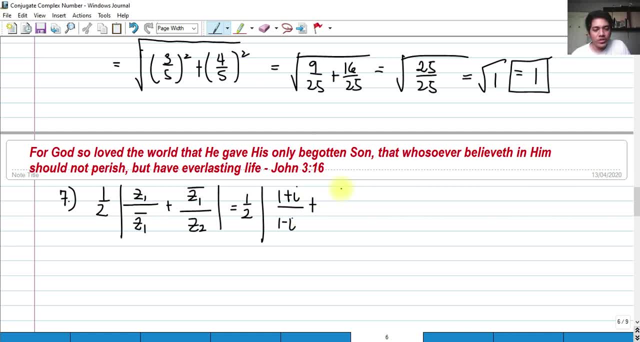 Okay, that is plus z sub 1, conjugate is 1 minus i, all over z sub 2.. Our z sub 2 is 2 minus 2i. Okay, so first, what we need to do is to evaluate first. 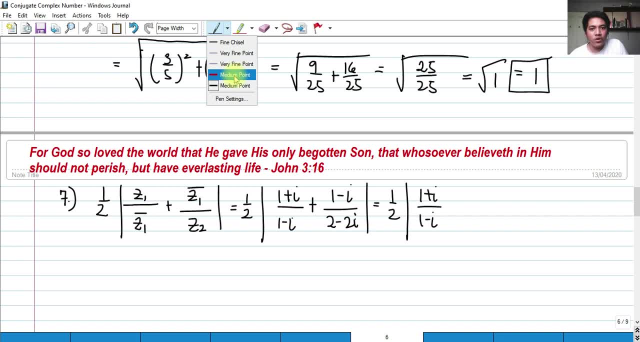 the first term. okay. multiply it by its conjugate denominator's conjugate: 1 plus i, 1 plus i, and that is plus 1 minus i, all over 2 minus 2i. okay, Okay, and we multiply it by the conjugate. 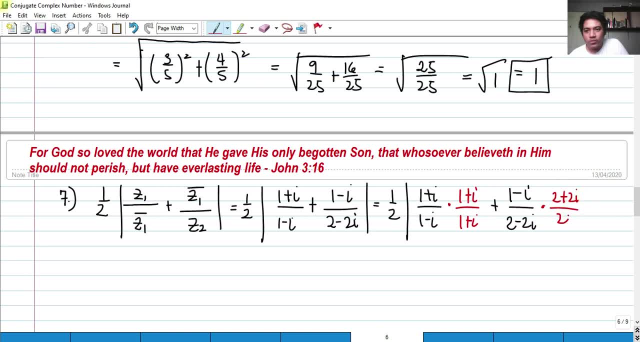 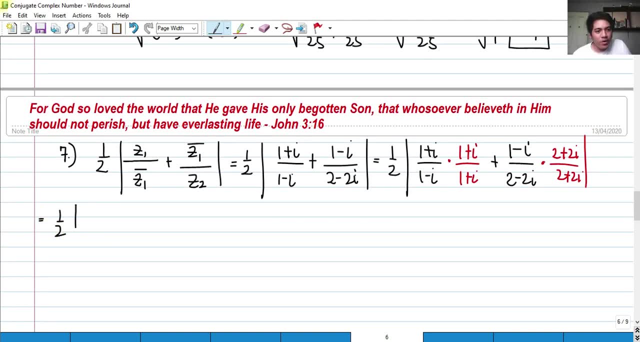 conjugate of the denominator 2 plus 2i. 2 plus 2i. okay. So what we're going to do, simply evaluate. so 1 half the modulus of we have 1 plus 2i, plus i squared. 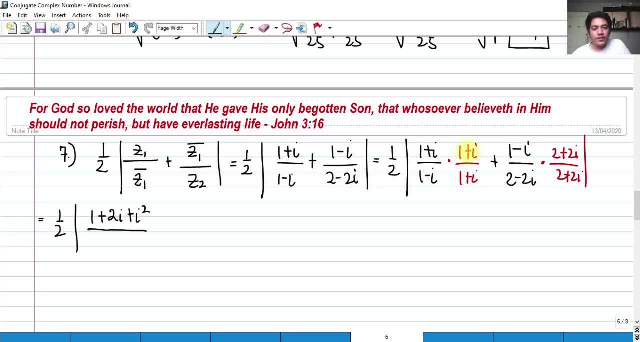 If we do this, okay, they are entirely the same. So we can have the shortcut for FOI. So we have 1 minus i times 1 plus i. that's 1 minus i squared Plus. we have to perform FOI on this. 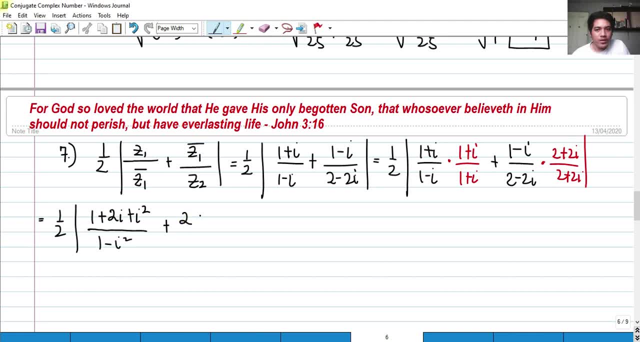 The first, the outer, would be plus 2i. inner, would be negative. i times 2,. that's minus 2i. and the last would be negative i times 2i. that's plus or minus 2i squared, Minus 2i squared. 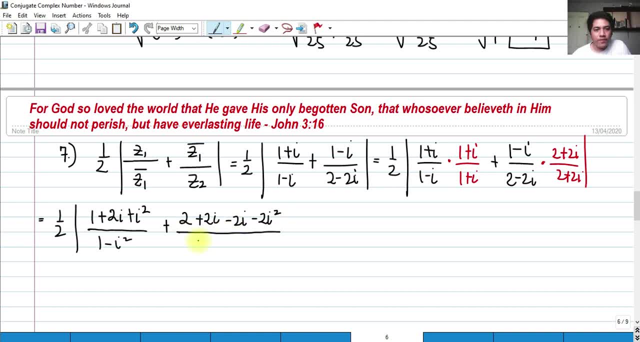 Okay, then all over, we have 4, minus 4i squared. take the modulus of that. Okay, so evaluate this: we have 1 half, okay, 1, that's 1 half multiplied by the modulus. 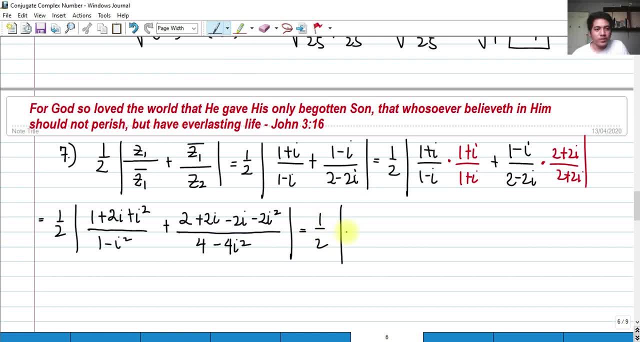 Oops, multiplied by the modulus. So we have: we know that this i squared is equal to negative 1.. So it's positive positive times. negative would be negative. so this is negative 1, plus 1,. we know that this 2 would cancel 1 minus 1, okay. 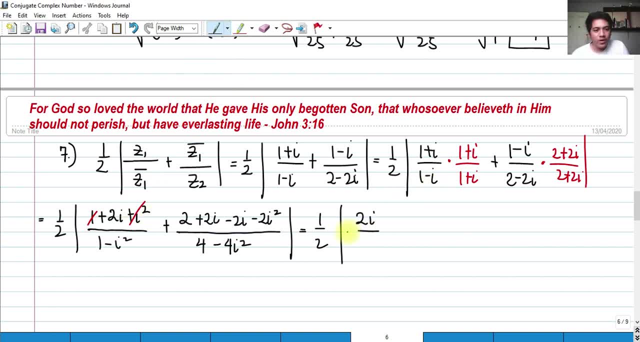 So, leaving 2i: okay, And we know that this should be 1 minus negative, 1, okay, That is plus. of course, we can also simplify: 2i minus 2i, positive, 2i minus 2i, that's 0.. 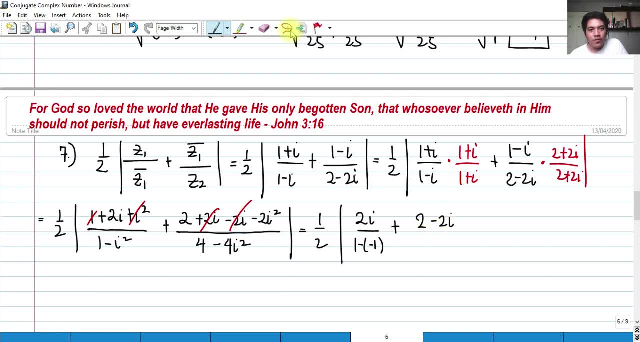 So we are left with 2 minus 2i, or 2 times negative 1, because i squared is equal to negative 1.. Negative 1, all over 4 minus 4 times negative 1.. So we have 1- half the modulus of 2i- all over 2.. 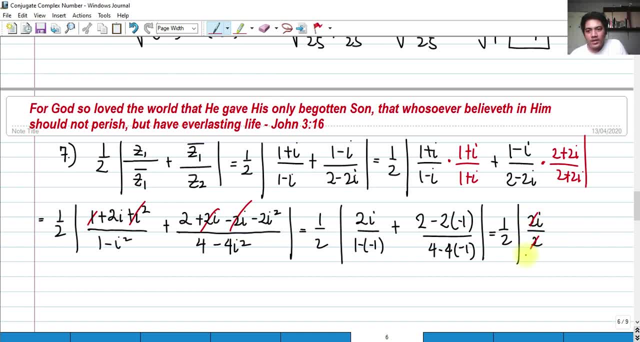 These 2s will cancel, okay, Cancel. so we have an i for the first term. So we have negative 2 times negative 1, that's positive 2.. So positive 2 times plus positive 2, that's 4.. 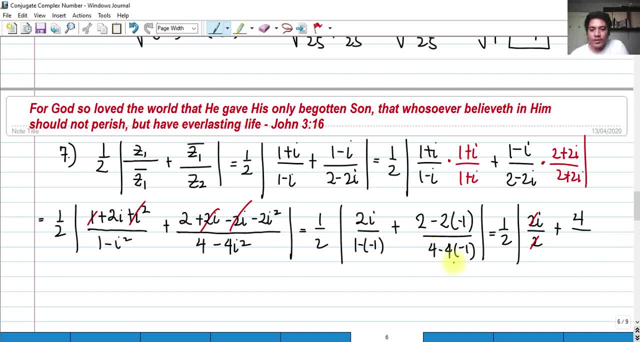 All over we have negative 2, plus positive 2,, that's 4.. All over we have negative 4 times negative. 1, is 4.. 4 plus 4 is 8.. Okay, so we have 1, half the modulus of i. 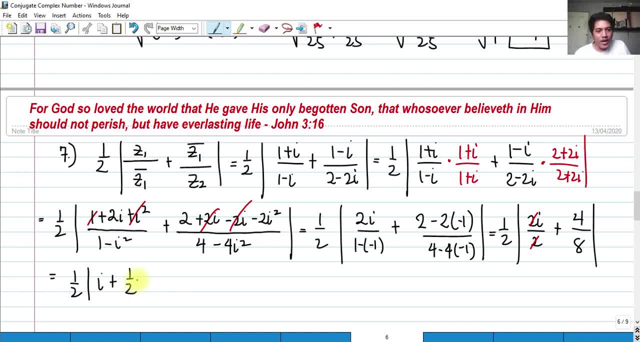 We can reduce this into lowest term. we have 1 half, So we perform that. how are we going to write this? We have 2i plus 1 over 2, okay, Modulus of that. So in other words, we have 1 half. 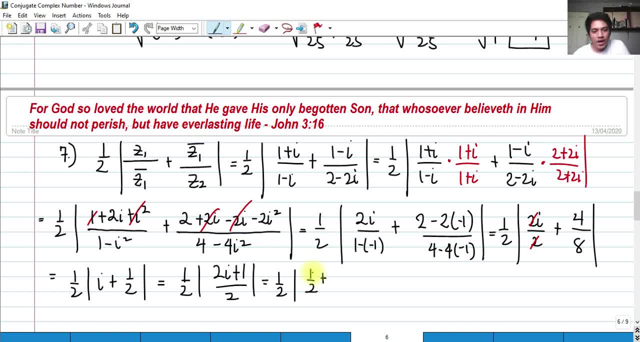 the modulus of. we can rewrite this as 1 half plus okay, plus i. It's still the same here- okay? So we need to get the modulus of this before multiplying by 1 half. So the modulus of this would be: 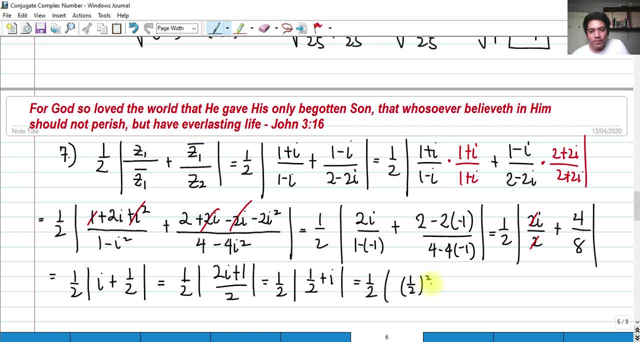 this term would be 1 half squared plus 1 squared. okay, Our x here is 1 half, our y here is 1.. So hence we have 1.. So if we're going to multiply that, evaluate that that is 1 fourth plus 1, okay. 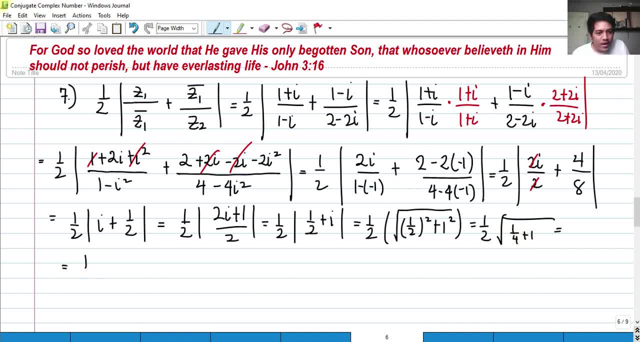 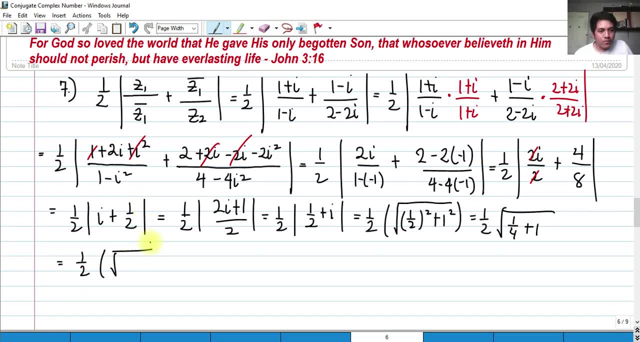 So we know that this would be equal to 1 half multiplied by the square root of 5 over 4.. Okay, and then we can evaluate this as we have square root of 5, okay Over 4.. Over square root of 4.. 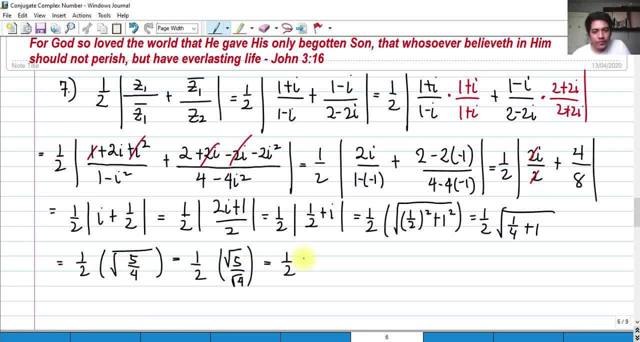 That's the same with this. So we have 1 half square root of 5 over 2, okay, Because we can evaluate square root of 4 as 2.. So we have square root of 5 over 4.. So that is our answer for this problem. 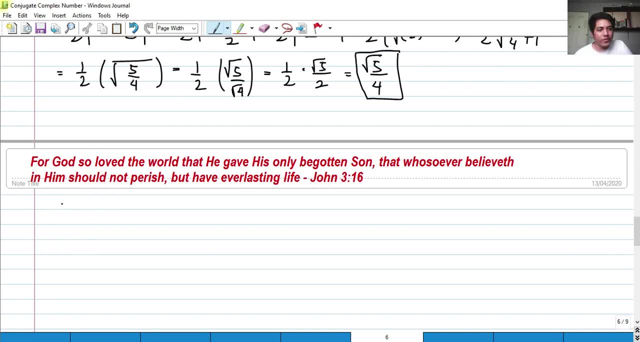 And as for our last problem for today's video, so we have number 8. We have the modulus of the conjugate of j sub 1 multiplied by j sub 2, plus we have i j sub 1, minus i j sub 2. 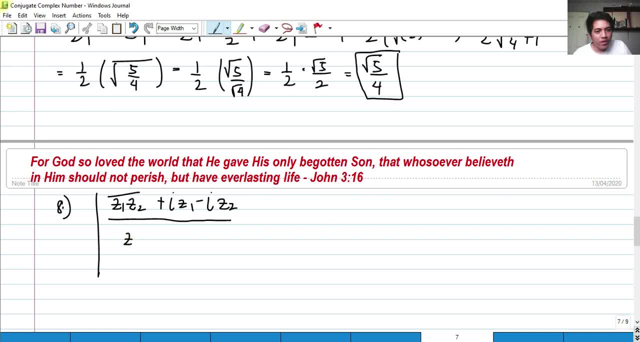 all over the conjugate of the sum of j sub 1 and j sub 2.. So this is j sub 2.. Oops, Let me just rewrite this: j sub 1 plus j sub 2.. Then we have plus, okay. 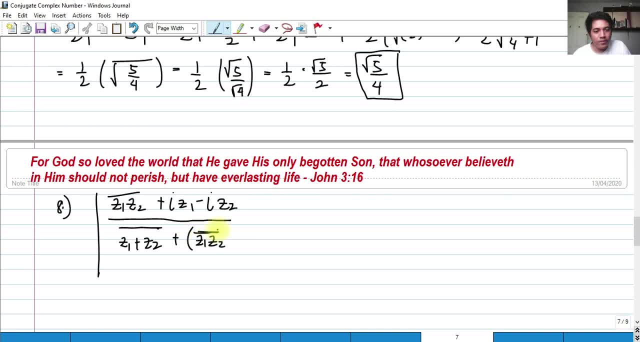 the conjugate of the product of j sub 1 and j sub 2.. So what are we going to do is we can use the properties of conjugate here, This one, the product of the, the conjugate of the product of j sub 1 and j sub 2. 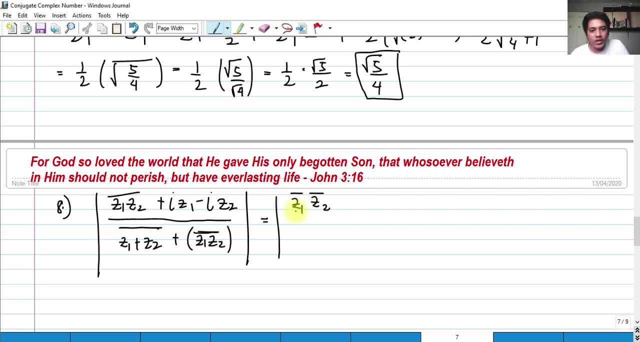 can be written as individually: the conjugate of j sub 1 multiplied by j sub 2.. So we have j sub 1 plus i j sub 1 minus i j sub 2. all over we have j sub 1.. This could be also rewritten as j sub 1,. 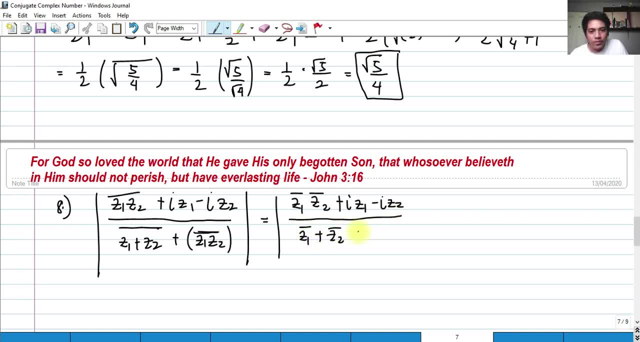 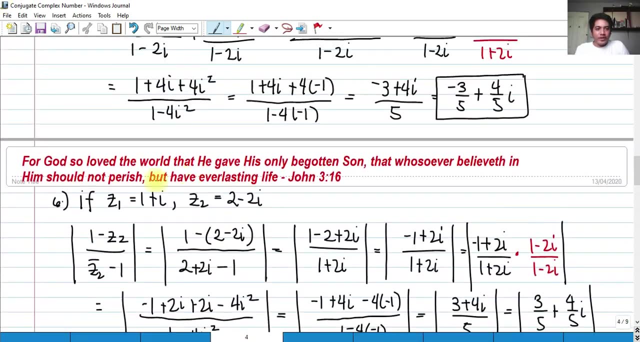 the conjugate of j sub 1, plus the conjugate of j sub 2, plus we have conjugate of j sub 1 multiplied by conjugate of j sub 2.. And don't forget the modulus. So the modulus is should be our final answer here. 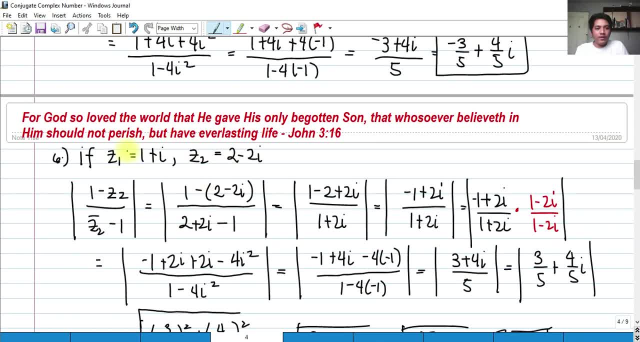 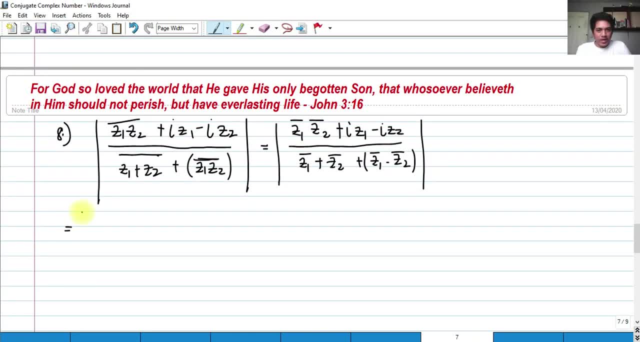 So it should be a real number. So, taking back in our given i plus 1,, 2 minus 2i. Let's take a look back. So we need to substitute that. Okay, we need to substitute our values. So what are we going to do? 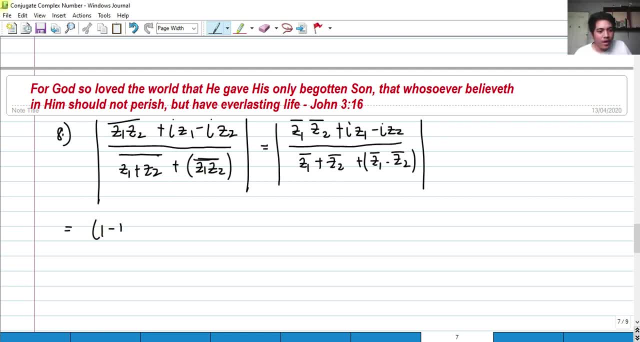 We have j sub 1, the conjugate of that, that is 1 minus i. Conjugate of j sub 2, that is 2 plus 2i plus i times j sub 1, which is 1 plus i. 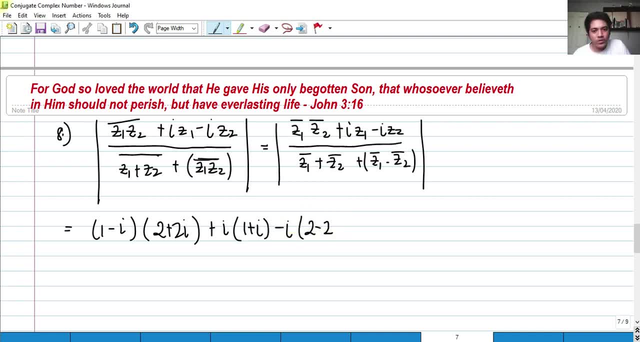 minus 2i, Okay, all over. conjugate of j sub 1, that is 1 minus i, okay. plus. conjugate of j sub 2, that's 2 plus 2i, okay, and then plus, okay, the same thing here: 1 minus i multiplied. 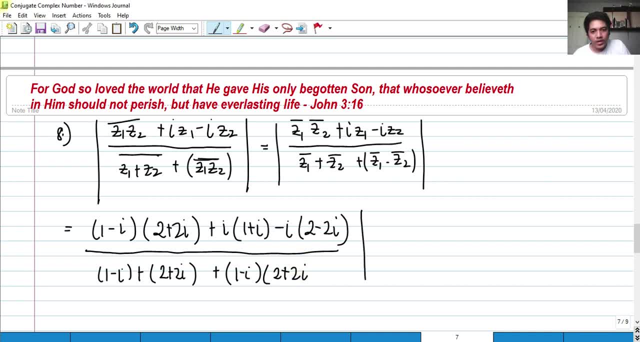 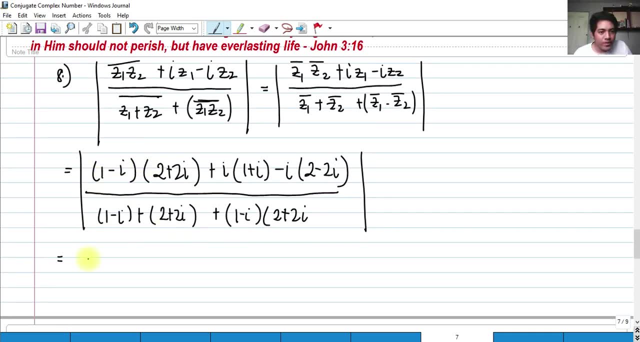 by the conjugate of j, sub 2.. Of course, don't forget the modulus. Okay, So what are we going to solve this? So, if we solve this, we have Coyle method. So the first one would be 2, outer would be plus 2i, inner would be negative 2i. then 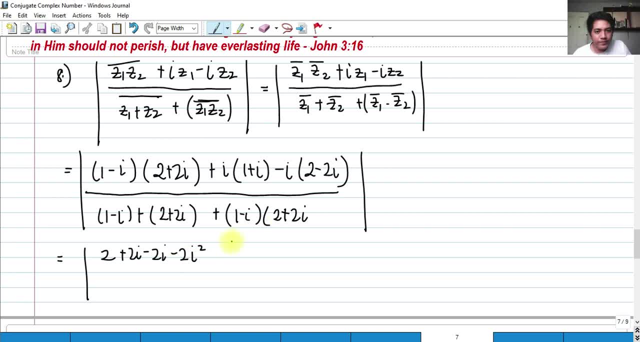 last would be minus 2i squared plus. we need to distribute this. this would be i plus i squared. and the last one: here we need to distribute i together with its sign, because that is a minus. So we have negative 2i minus or plus 2i squared negative times: negative would become plus. 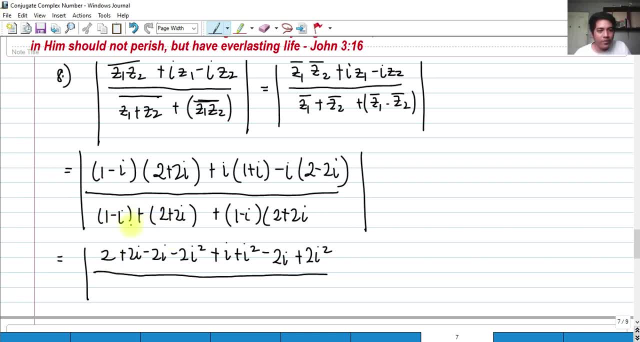 Okay, Then on the denominator we can have, we can add this: okay, first. no, we can add this, So we have 1 plus 2, that's 3, minus i plus 2i, that's plus i. then that is added to the. 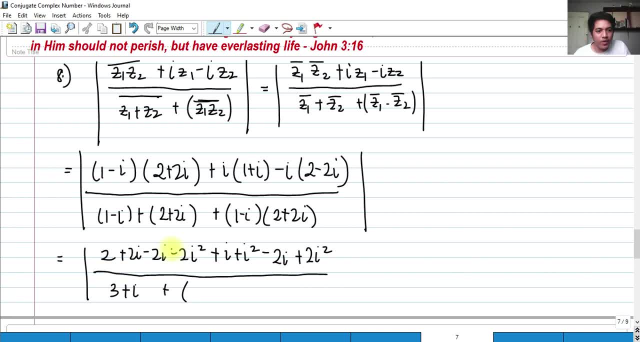 sum of this. So which is this? This is the same to this one, So we have 2 plus 2i minus 2i minus 2i squared. Take the modulus of that. So, as you can see here, we can cancel this okay. 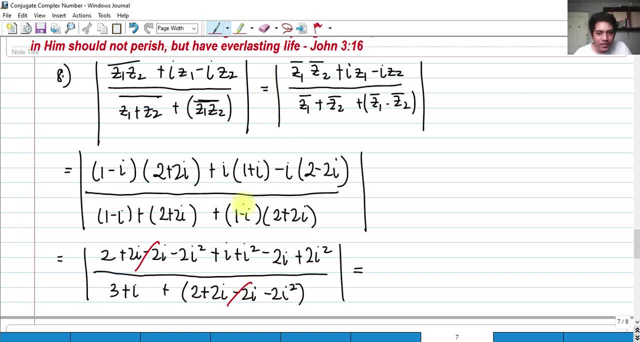 That would be zero. Okay, Is there anyone else? Negative 2i squared: okay, we have plus 2i squared. could be canceled. okay, So, and we evaluate it, So let's try. So we have the modulus of 2,, okay, 2.. 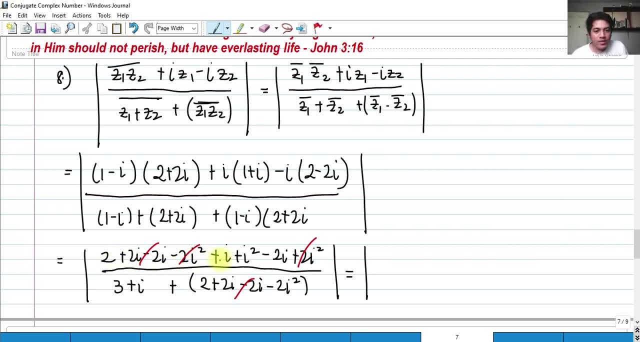 So what we're going to have here- 2 plus we have this is- would become negative 1.. So 2 minus 1 would be 1.. Then we have: plus i minus 2i would be minus i and for our denominator, of course, we. 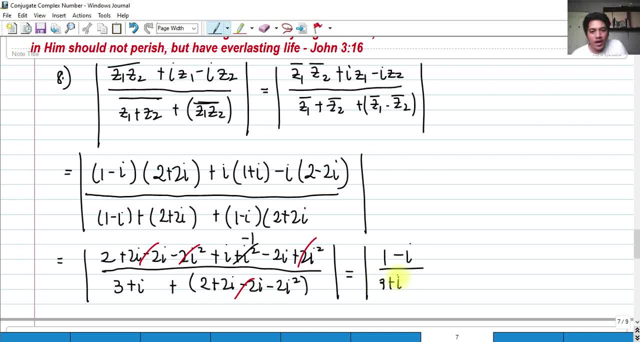 have 3 plus i, Then we have 2i. Okay. Then we have plus 2, okay. minus 2 times negative 1 because of i squared. So we have 1 minus i. all over 3 plus 2 is 5, okay. 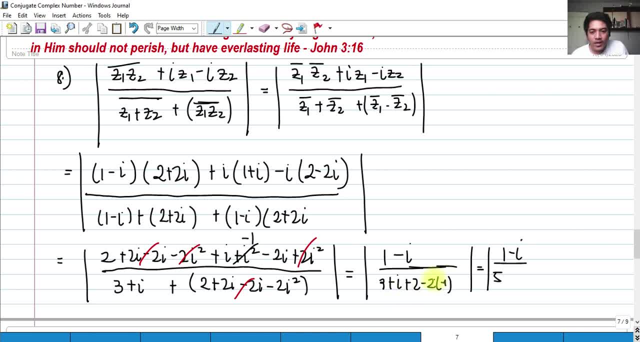 And then we have 2 times negative, 2 times negative, 1, that is plus 2. And then we have plus i. So we have 1 minus i all over 3.. We have 1 minus i all over 7, plus i. 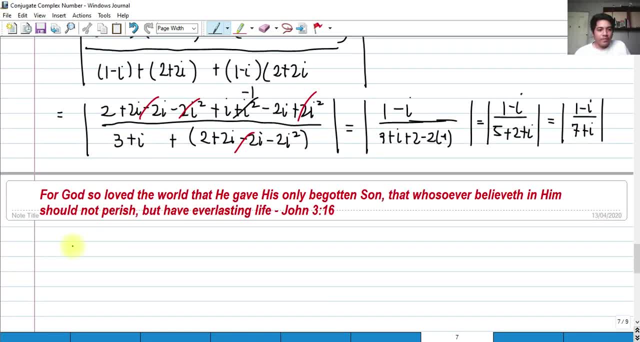 So get the modulus of that, Okay, But before we get the modulus of that again, we need to solve it by multiplying the whole equation by the conjugate of its denominator. Let me just rewrite this: So we have 1 minus i, all over 7 plus i, multiplied by the conjugate of the denominator. 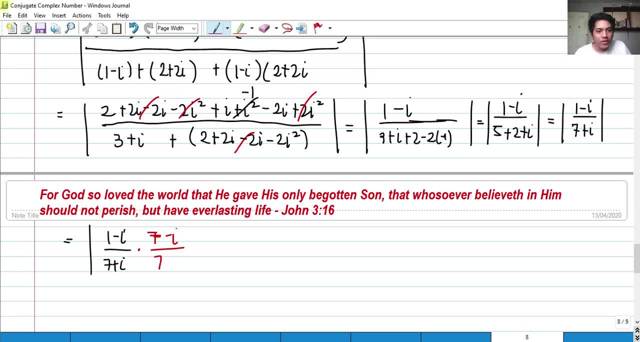 So we have 7 multiplied by 7 minus i, All over 7 plus i. Okay, 7 minus I. and of course it's modulus. don't forget the modulus. so we have first 1 times 7, outer negative I times 1, that's minus I, inner minus 7 I last we. 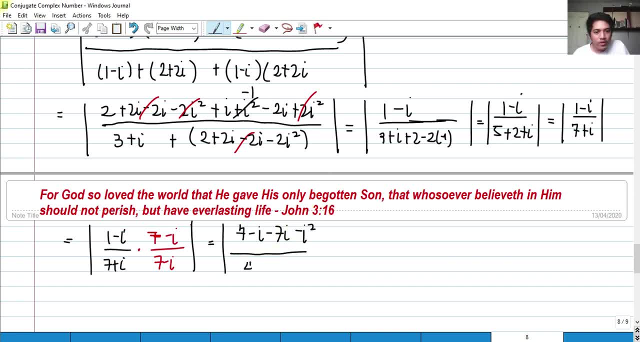 have negative. I squared all over 49. okay, minus I squared, so this would be 7 or this would be positive 1 I squared, so we have. let me just rewrite: 7 minus 7, I okay, 7 negative I minus 7 I, that's negative, 8 I. then we have negative times. 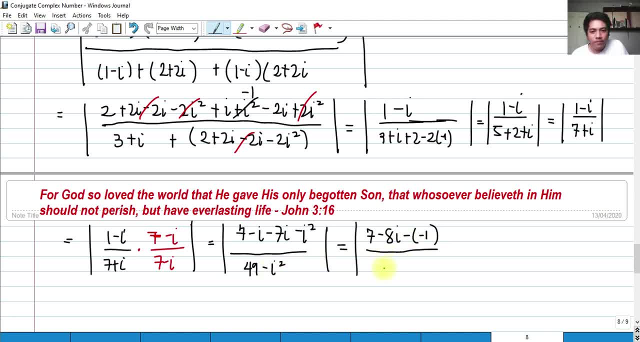 negative 1 minus times negative 1. this would become 49 minus times negative 1. so we have: well, of course, this should be positive. my mistake, okay, this should be positive, because negative items device would be positive. I squared. okay, so we have 7 minus 1. that should be 6. 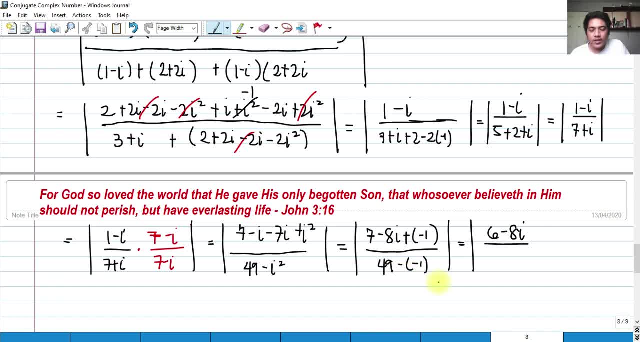 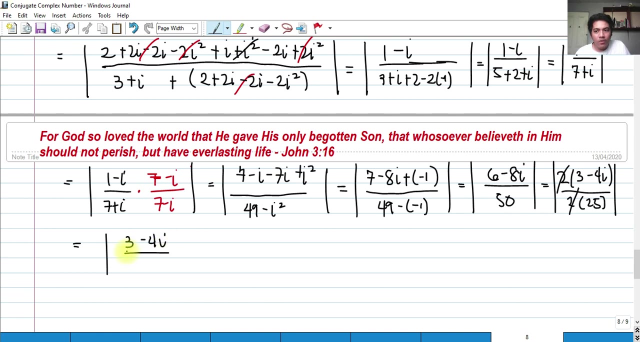 minus 8, I all over 49. minus negative 1, we have 50. then we can proper out 2. okay, 3 minus 4, I all over 2 times 25. we can see that the twos would cannot, And so, and then we have, finally we have, the modulus of 3 minus 4i- all over 25.. 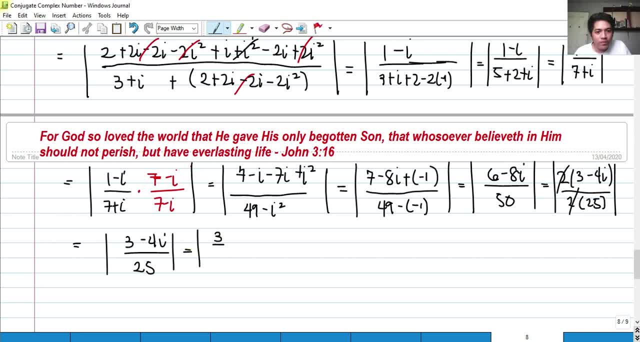 So we can have now as modulus of 3 over 25 minus 4 over 25i. So if we get the modulus of that, so we have 3 over 25 squared plus we have negative 4 over 25 squared, taking the square root of that. 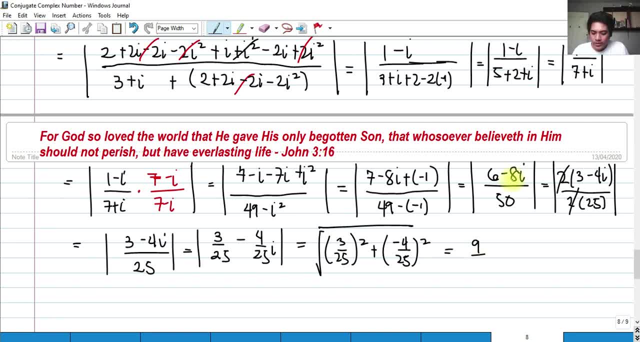 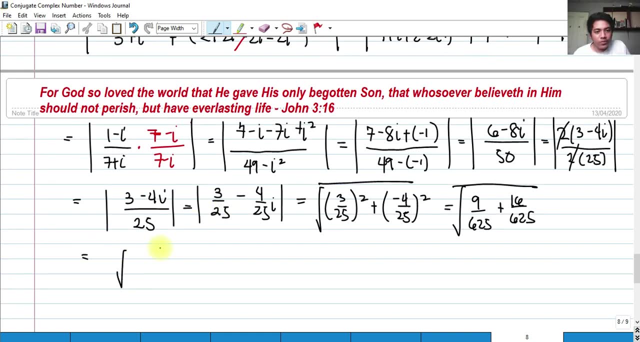 So we have 9 over 25. squared is equal to 625.. So we have 625 plus 16 over 625 and then we have the square root. So we have square root of 25 over 625 and if we evaluate that, simplify the fraction inside. 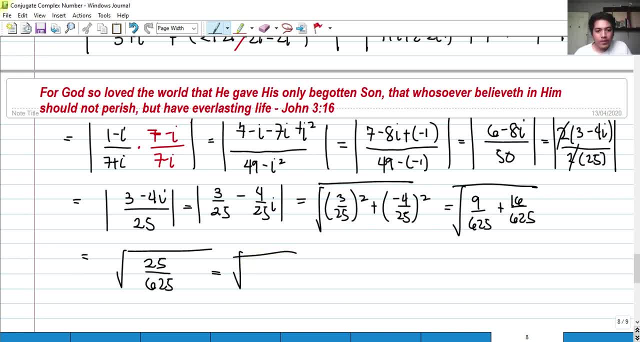 we have 1 over 25 by the square root. we have this one. our answer should be 1. fifth. So that's the modulus for our problem number 10.. Okay, so, thank you so much for listening. Don't forget to subscribe on my YouTube channel if you are new to my YouTube channel.